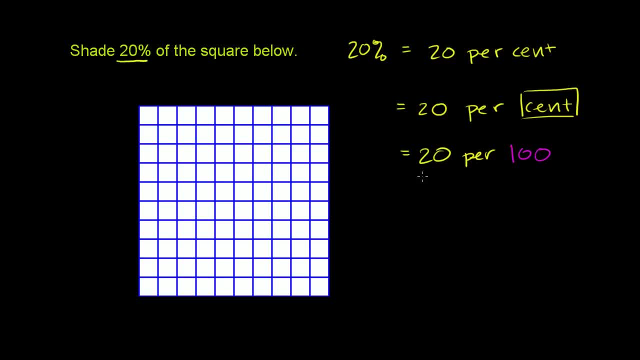 square into 100 pieces. we want to shade the square. We want to shade 20 of them, 20 per hundred. So how many squares have they drawn here? So let's see, if we go horizontally right here, we have 1,, 2,, 3,, 4,, 5,, 6,, 7,, 8,, 9, 10 squares. 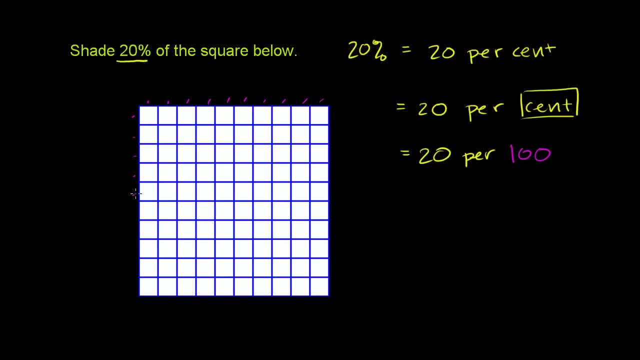 If we go vertically, we have 1,, 2,, 3,, 4,, 5,, 6,, 7,, 8,, 9, 10.. So this is a 10 by 10 square, So it has 100 squares, here. 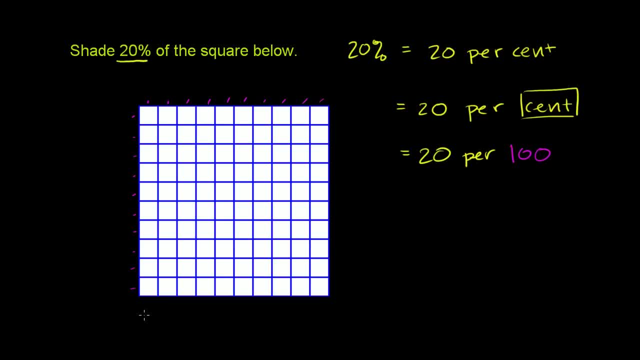 So if we want to shade this or another way to say it, is that this larger square- I guess that's the square that they're talking about- This larger square is broken up into 100 smaller squares, So it's already broken up into the 100.. 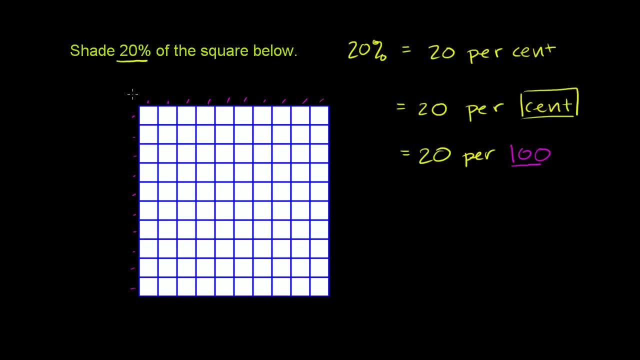 So if we want to shade 20% of that, we need to shade 20 of every 100 squares that it is broken into. So in this we'll just literally shade in 20 squares. So let me just do 1.. 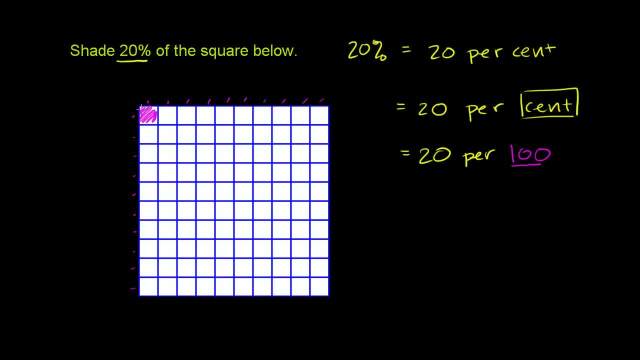 So if I just do 1 square just like that, I have just shaded 1 per 100 of the squares. 100 out of 100 would be the whole. I've shaved 1 of them. This would be that 1 square by itself would be 1% of the. 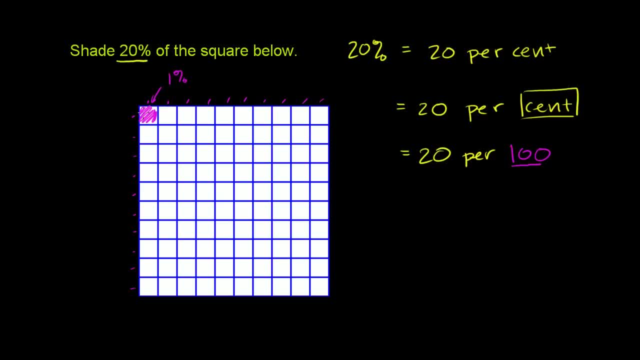 entire square. If I were to shade another one, if I were to shade that and that, then those two combined that's 2% of the entire square. It's literally 2 per 100, where 100 would be the entire square. 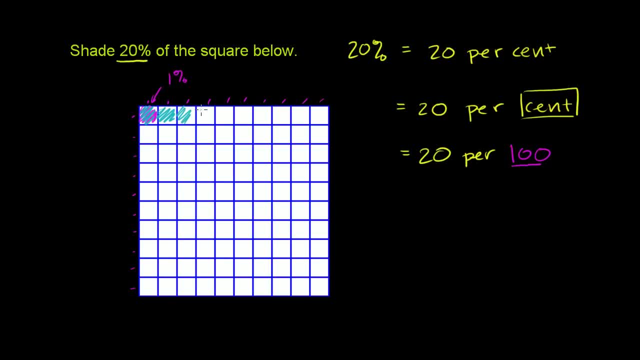 So if we wanted to do 20,, we do 1,, 2,, 3,, 4.. Actually, if we shade this entire row, that will be 1,, 2,, 3,, 4,, 5,, 6,, 7,, 8,, 9,, 10.. 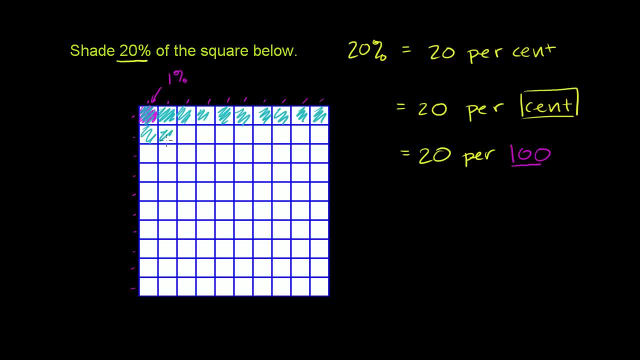 And then we want to do 20, so that'll be one more row, So I can shade in this whole other row right here, And then I would have shaded in 20 of the 100 squares, Or another way of thinking about it. if you take this. 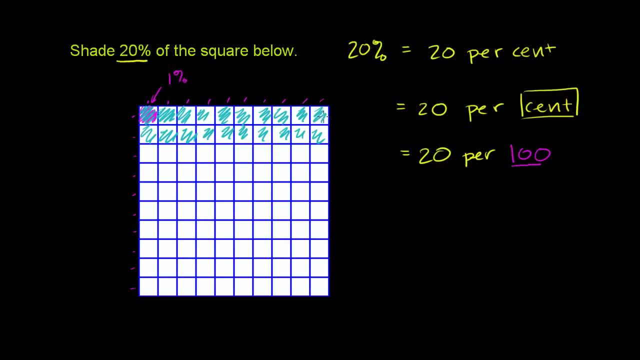 larger square. divide it into 100 equal pieces. I've shaded in 100, or I've shaded in 20 per 100, or 20% of the entire square. Hopefully that entire larger square. hopefully that makes sense.